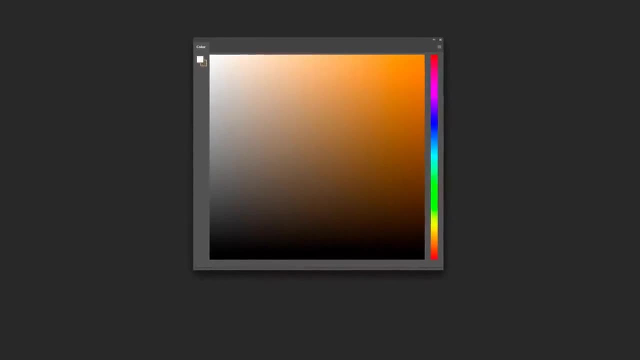 Today on Quick Essentials, I want to show you an odd little thing you need to know about color. This kind of blew my mind when I first learned about it. First, though, there are three terms we need to be familiar with. This area of the color picker is where you select your hue. 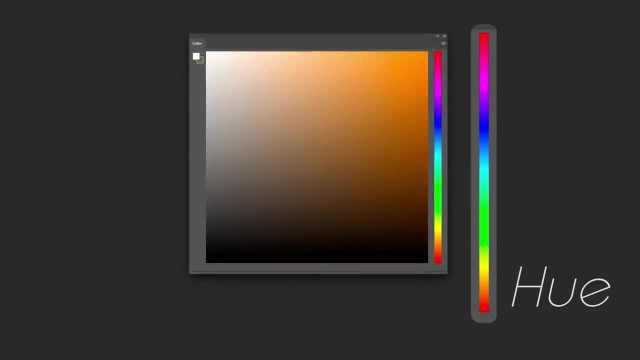 Hue is just the color name: red, green, blue, etc. Going horizontally across the color picker is how you select saturation. Saturation is the amount of chroma or intensity of a color, And going vertically like this will affect value. Value is how light or dark a color is. 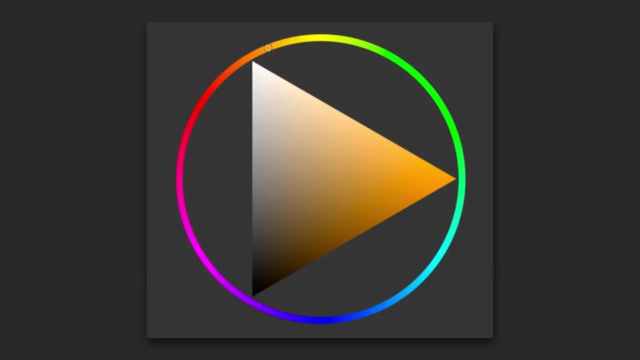 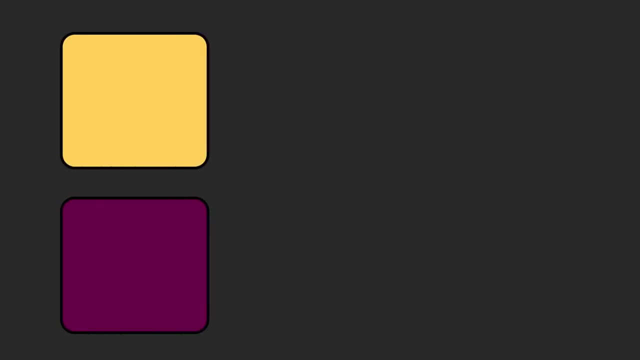 Some color pickers look like this, which is largely the same thing, although there are some implications we'll look at later in this video. Okay, so a color is always tied to a value, Even though these are two different hues with two different levels of saturation. 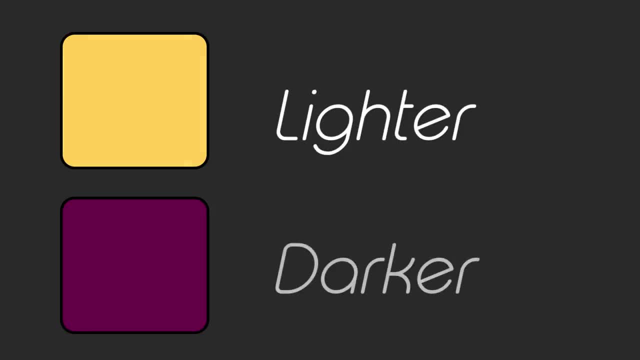 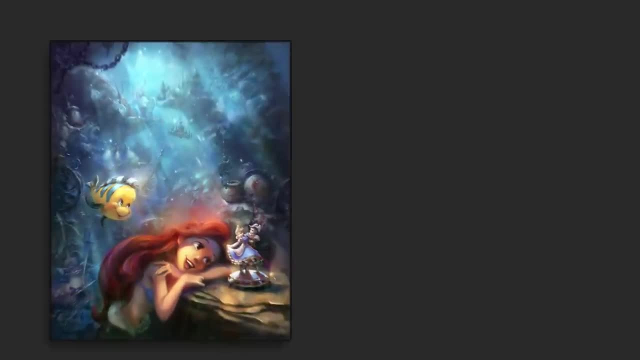 I think it's pretty easy to see that the top one is lighter and the bottom one is darker And, stripping away the saturation, we can see exactly where the values of those two colors lie, And because it's value, not color, that makes a picture readable. 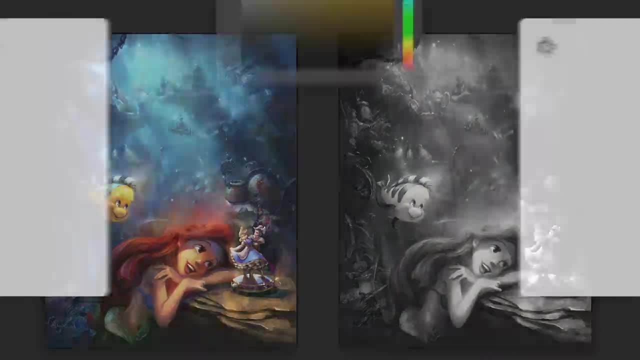 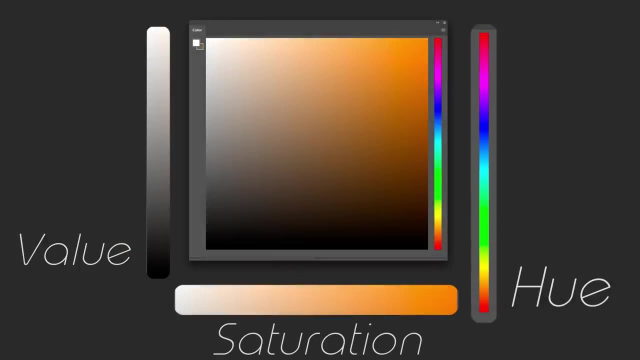 value is one of the most important fundamentals of painting. No matter what you do with hue and saturation, your decisions there always boil down to value. Now, it's very tempting to think that hue and saturation are independent of value. You know like value is determined by this vertical. 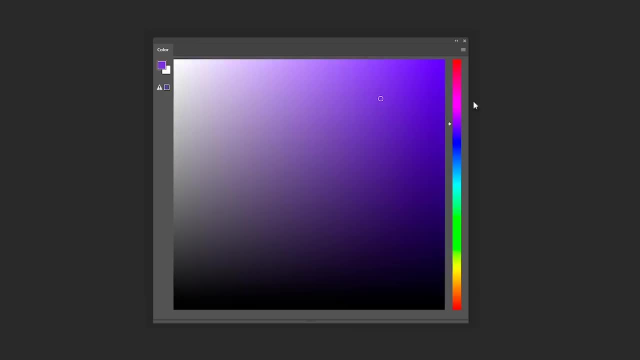 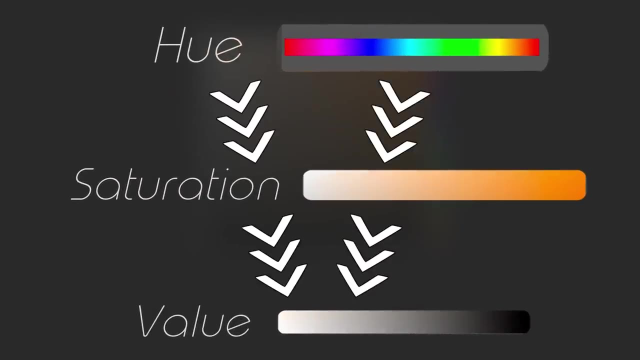 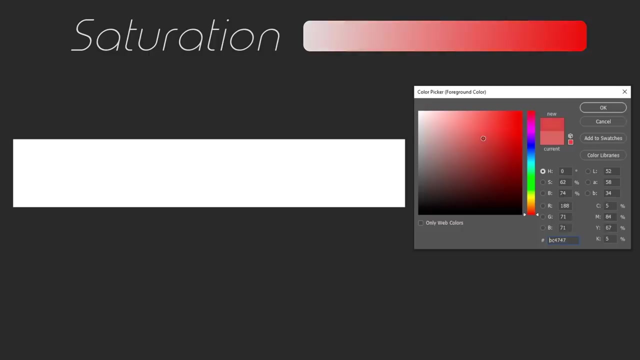 placement, and then you plug in hue and saturation after. But that is actually quite far from the truth. In fact, every single aspect of your color choices cascades down and affects value. I'll show you an example with saturation first. Here's a color picker and a canvas. I'll use this red hue here. I'll start with a perfectly 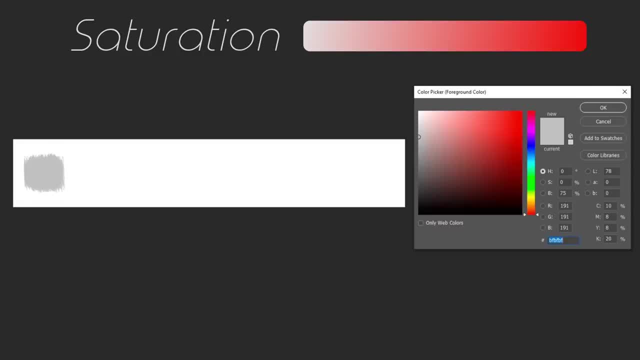 desaturated version of that and paint a little swatch. Now I want to increase the saturation while staying at the same brightness level on the color picker. So here's another swatch. change the saturation level- here's another swatch- and repeat this process all the way to the end. 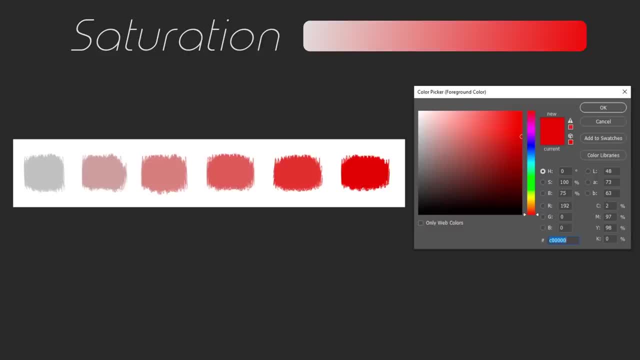 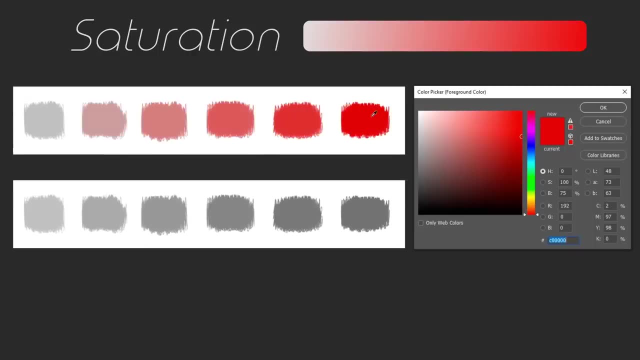 Okay, now check this out. I'm going to convert this to black and white And the values are different: Adding saturation, decreased value, Even though, as I sample these, Photoshop is telling me I'm at the same brightness level Again. it was a straight line all the way across that color picker And that's where these 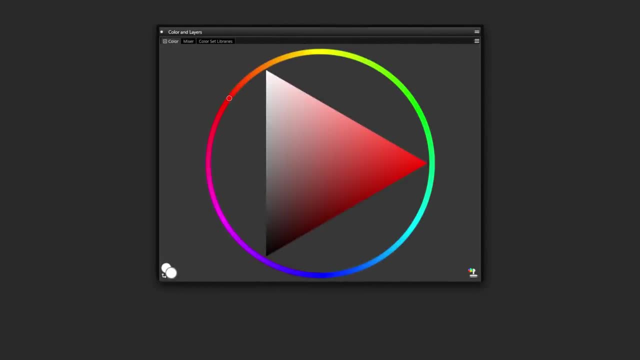 triangular pickers are a little bit more visually accurate. This is Corel Painter's color picker. by the way, Its shape implicitly tells us that this value is lighter than this value, And remember how Photoshop's brightness was not reflecting our value change On this color picker. 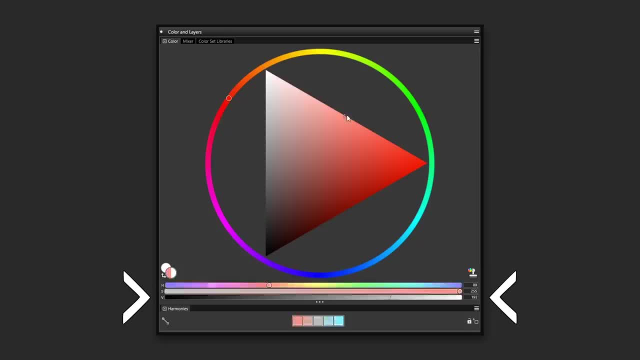 I'm going to apply a little more saturation to this value. I'll show you how. It's not totally accurate. I'll show you why in just a second. But first I want to point out that not all color pickers are made equal. This is Photoshop's Cooleris. 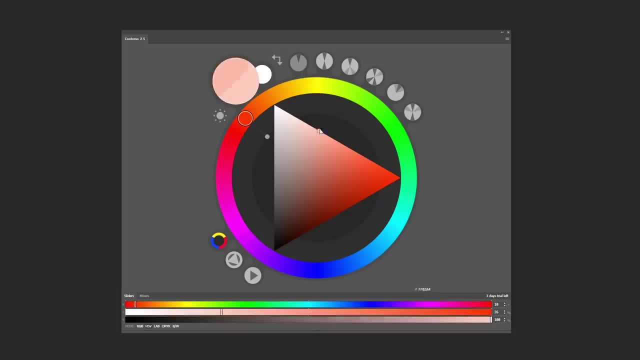 plugin, which is also a triangular picker, And I like this plugin, by the way. But here I am doing that same color move, but on this one the value slider stays locked at 100.. It's almost like different color pickers are measuring different properties. Okay, Time to. 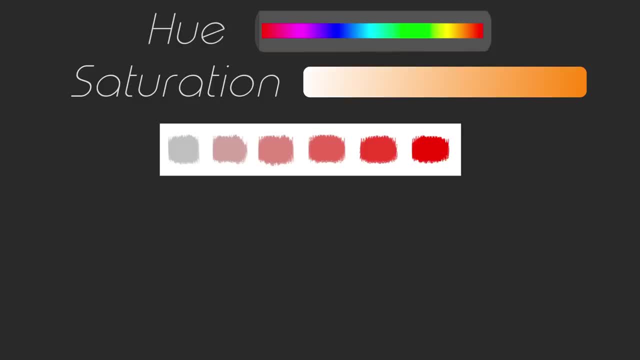 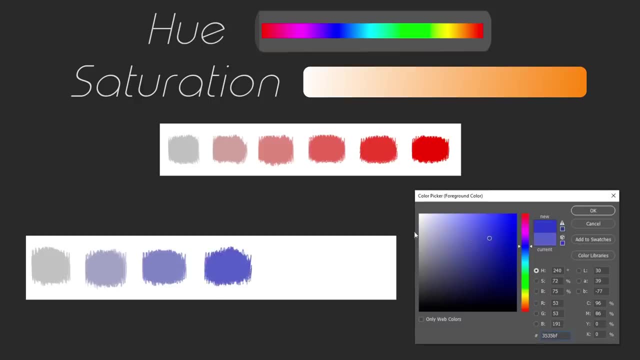 move on to how hue affects value, and this is what really blew my mind. So there's our example with red at the top, and I'm redoing the process now with this blue color, And I'm using the same brightness value on this blue as I did on the red. Okay, so there's our two swatch panels. Watch what? 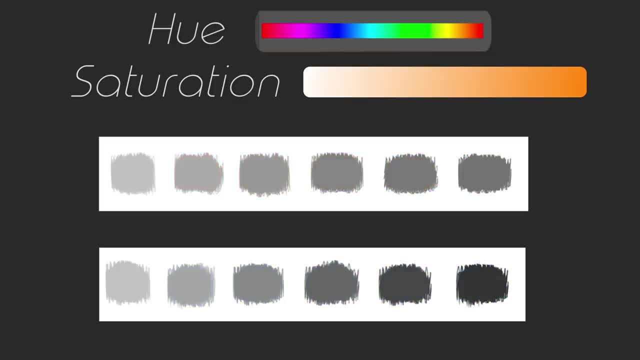 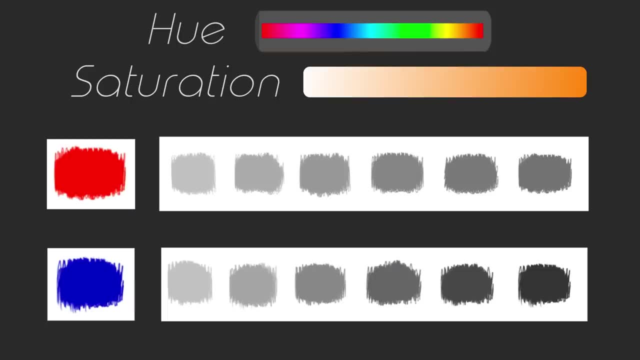 happens now as I switch this to grayscale. Your eyes do not deceive you. Different colors saturate to different values. This is a crucial piece in the puzzle of understanding color. It's also the source of some digital confusion. Back here in Painter, we've already seen how value does get. 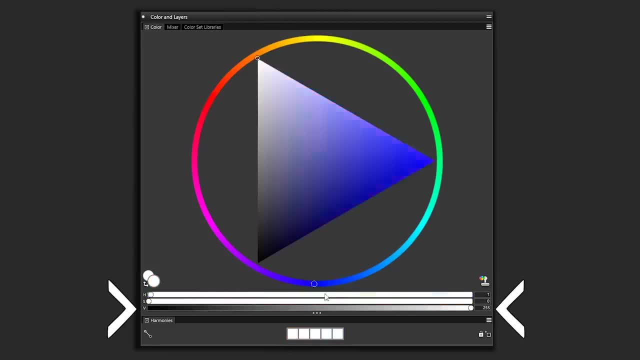 reduced as I make this move. however, the reason it's not entirely accurate is that Painter reduces the value of every hue equally, as we've just seen, that's not what actually occurs. In fact, check this out: Using this violet color, I'll pick a value right at 50%. on the grayscale I'll paint. 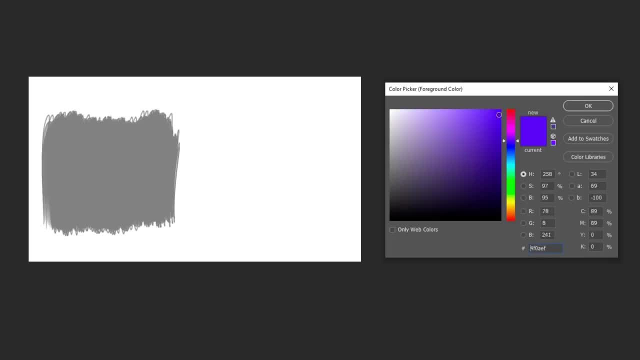 a swatch, and now I'll move the color picker up to full brightness, but also full saturation. Paint another swatch and are you ready? I'm gonna switch these to black and white. That is kind of crazy. We traveled halfway lighter on the. 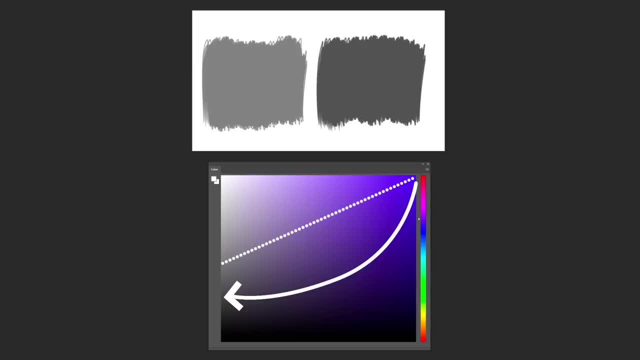 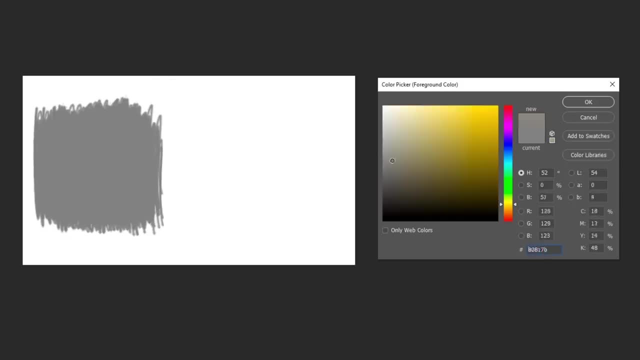 color picker and got a darker value. Lighter equals darker, dogs and cats living together. Now, this is not true for every color, of course. This yellow, for instance, does not get very dark when saturated. I've got my two swatches here. 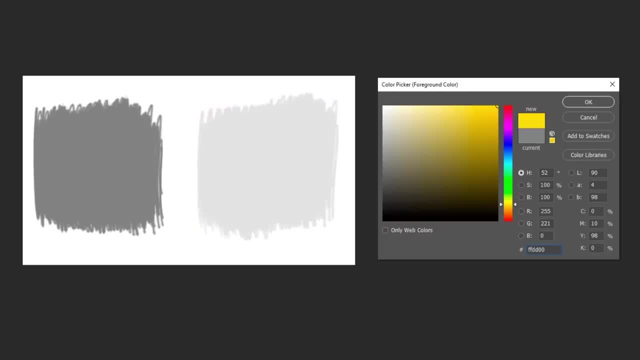 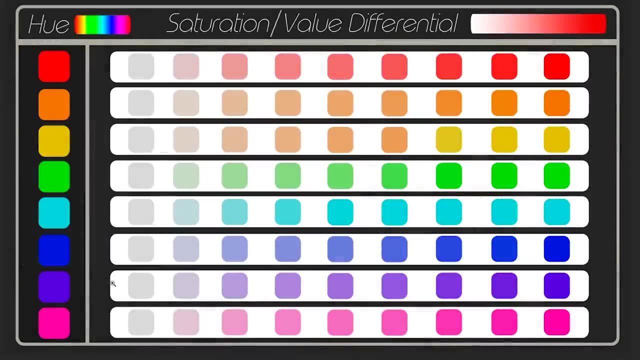 same as with the violet color, We switch to black and white, and this is more intuitive. Yep, that's the stuff that blew my mind, Okay, so I've made a chart for you to act as an overall reference for this. I've got it on two layers here: The 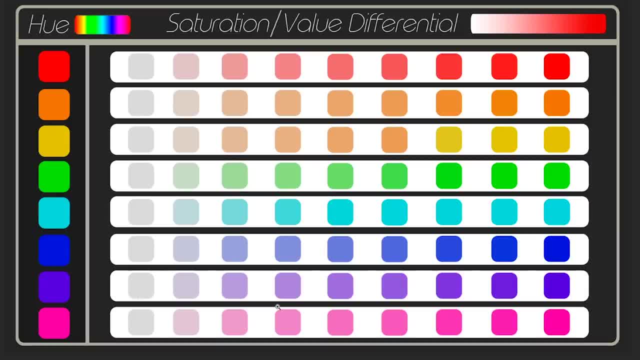 first layer is simply a chart with all the hues and various degrees of saturation, and then layer two, of course, is those saturation levels in grayscale, And this is not every granular hue change, but these, to me, are where the significant changes lie. You can find the download link in the description, So okay. 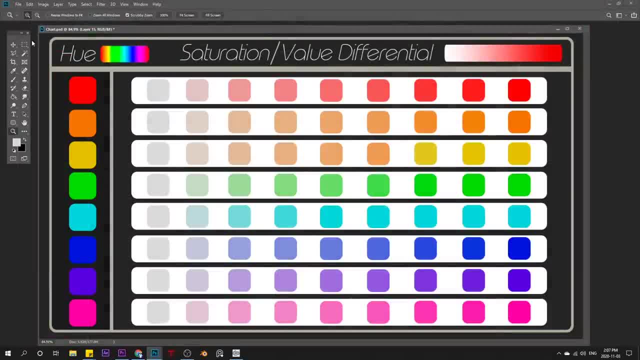 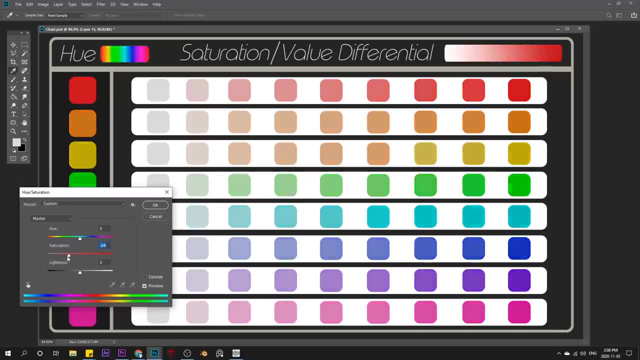 some more digital confusion. I'm afraid, Let's say, this represents a painting that I want to check in grayscale. The absolute wrong way to do it is to use the hue saturation adjustment. When I strip the saturation here, it just evenly levels everything out, which is 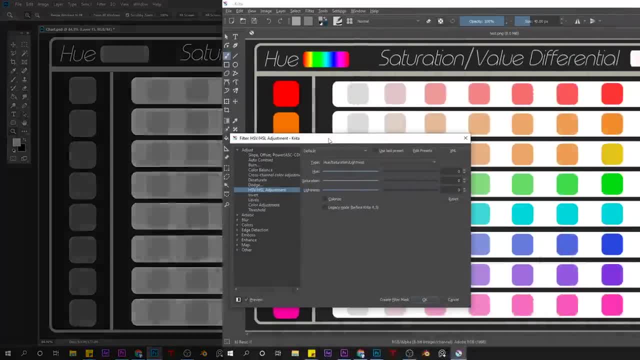 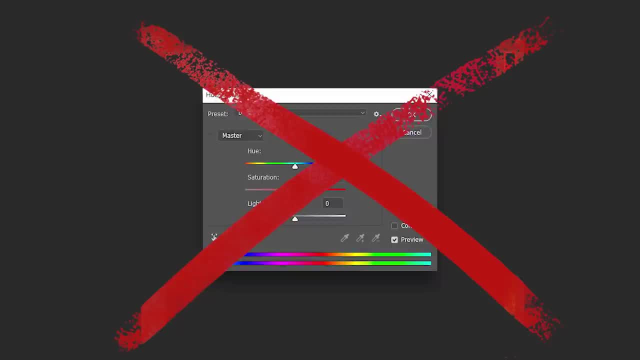 completely inaccurate. This is Photoshop, but the same thing happens in Krita, in Painter and in Clip Studio Paint. So don't use the hue saturation box to check values. One reliable way to do it is to simply switch the color space to. 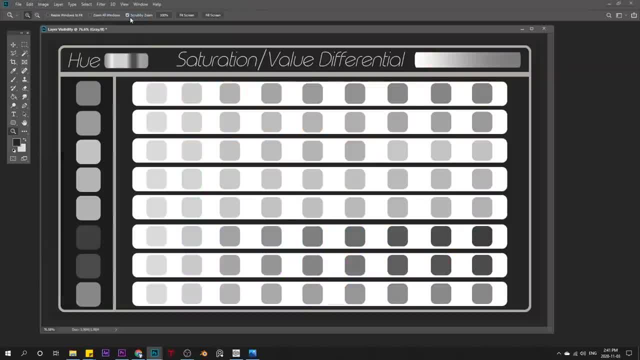 grayscale, but the drawback is in grayscale mode we can't paint in color anymore, so I usually don't do it that way. A quick and dirty way to do it is to make a new layer, fill it with white and then add a new layer. 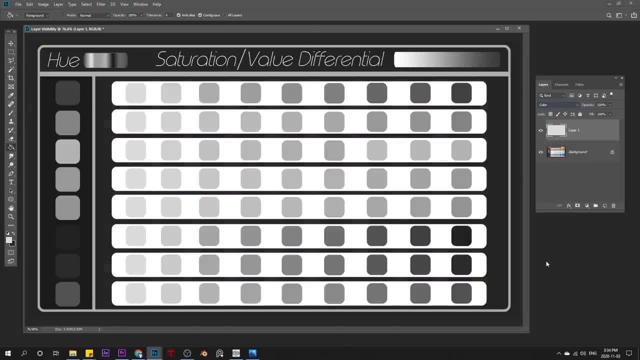 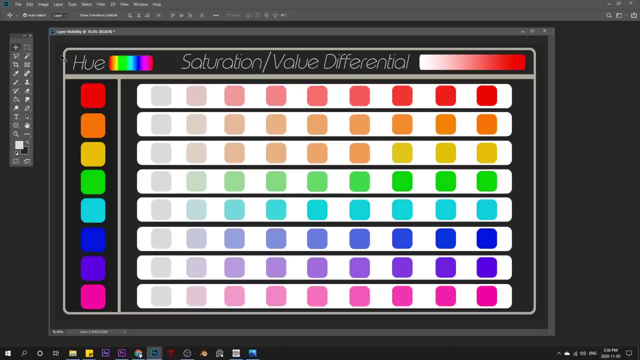 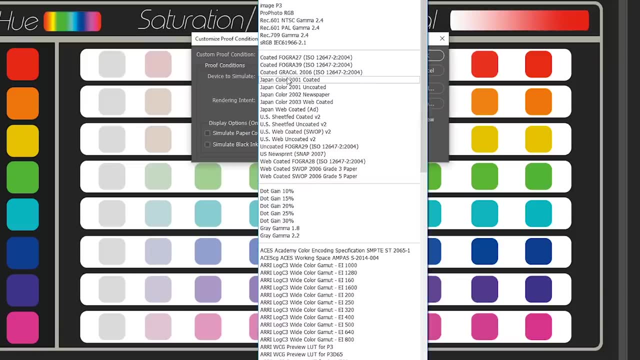 And set that layer to color mode. This works across multiple apps and it's pretty reliable, though I do think the contrast is exaggerated slightly. My favorite way to check values- and this is exclusive to Photoshop, unfortunately- go up to View Proof: Setup Custom. Then click the dropdown here and set it to. 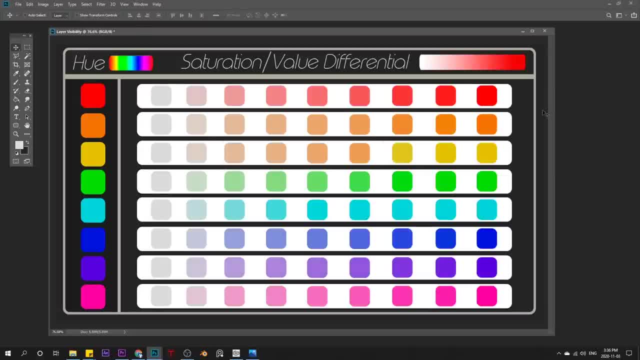 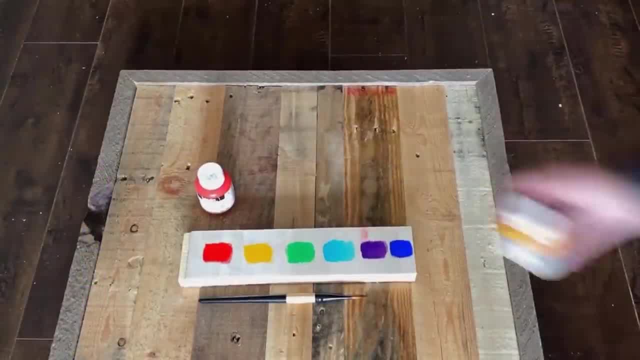 gain 20%. Now you can press control or command Y to toggle between an accurate grayscale view and color. And, by the way, this stuff happens with real pigments too. it's not just digital. Here are some swatches of these very bright and saturated acrylic pigments. 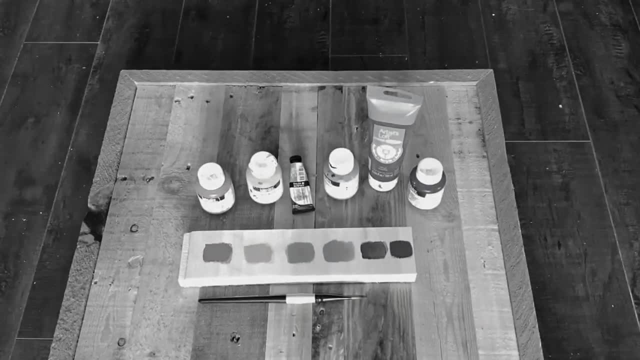 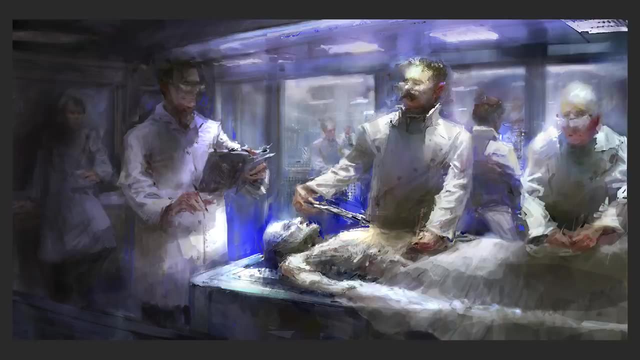 When I switch this frame to grayscale, we get the same value behavior Alright. I want to show you how this color theory actually influences my painting. Here's a spooky little sketch I did in October. There's a lot of grayish colors in it, so